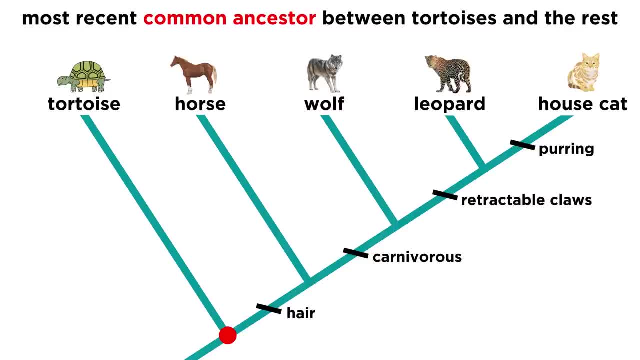 Like all animals, tortoises do share common ancestry with the other animals in the cladogram, the most recent of which is represented by this fork here, after which there is divergence. In fact, tortoises share many characteristics with mammals. They have an 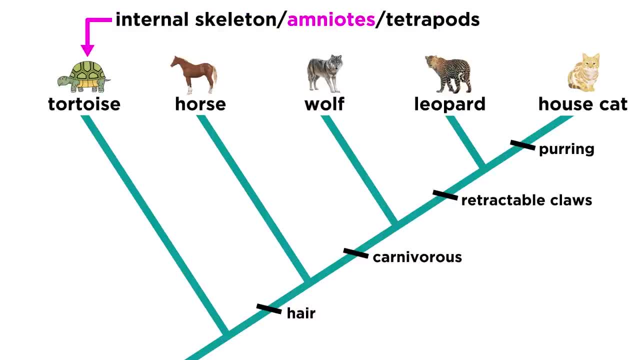 internal skeleton. they are amniotes that give birth to offspring on dry land. they are four-limbed tetrapods, and the list continues. However, we are not concerned with those shared characteristics in this particular cladogram. We are only interested in animals with hair. 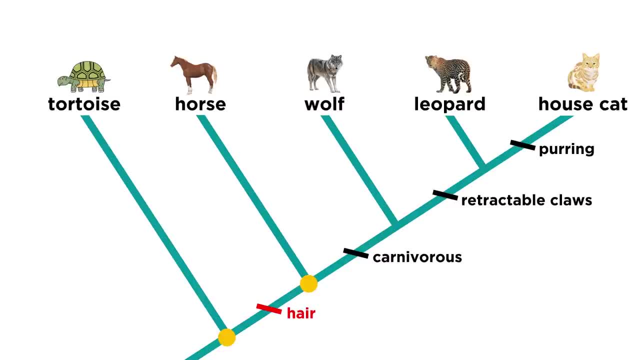 which are referred to as mammals. Again, since the word hair shows up right between the branches, leading to tortoises and horses, it means that this characteristic arose after the most recent common ancestry of these groups. There are no tortoises in existence. 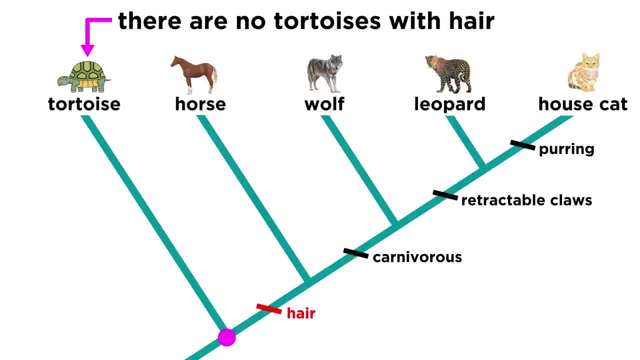 either extant or in the fossil record with hair. Since the hair characteristic is shared by all the animals in the study group, we call it an ancestral characteristic. All animals in the in-group share this characteristic. It is, in fact, an ancestral characteristic of all mammals. One quick note about ancestral characteristics. 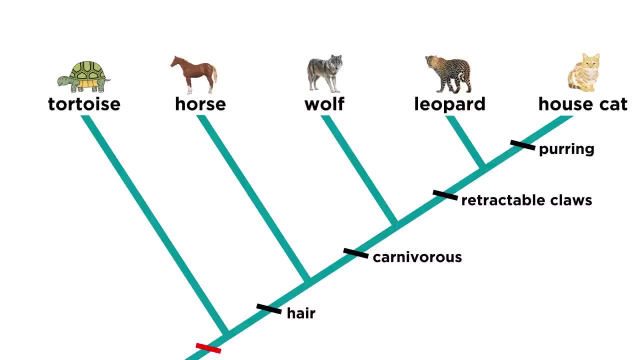 and outgroups. In some cladograms, the ancestral characteristic is placed at the very base. For example, we could have chosen backbone as the ancestral characteristic if we had preferred. As we will come to see, cladograms are simply concept maps. After the word hair, you'll then see the word carnivorous, The horse lineage branches. 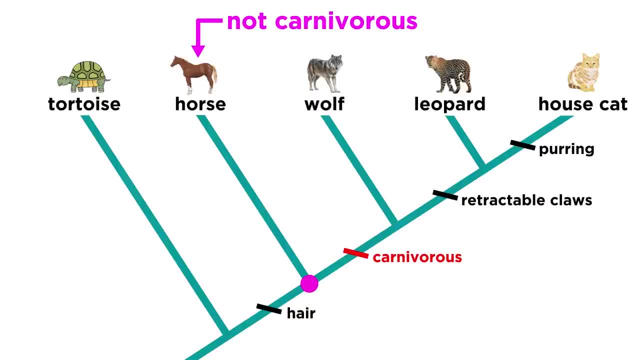 off here. This is because horses do not share that characteristic, That is, horses are not part of the mammalian order carnivora, as wolves are. However, horses do have hair, being members of mammalia, so horses are more closely related to wolves than tortoises. 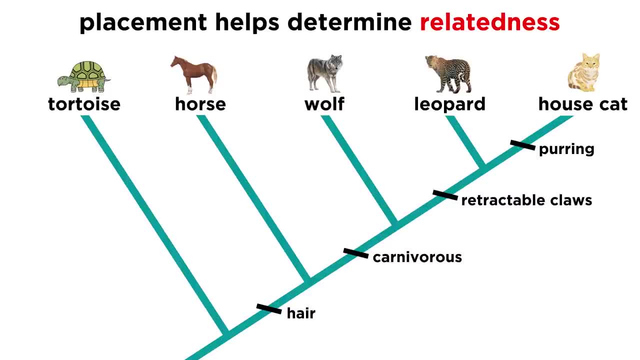 As we are beginning to understand. an animal's placement on a cladogram can help determine its relatedness to other animals. If we continue up the cladogram, we see that the wolf, for example, is more closely related to the leopard than to the horse. 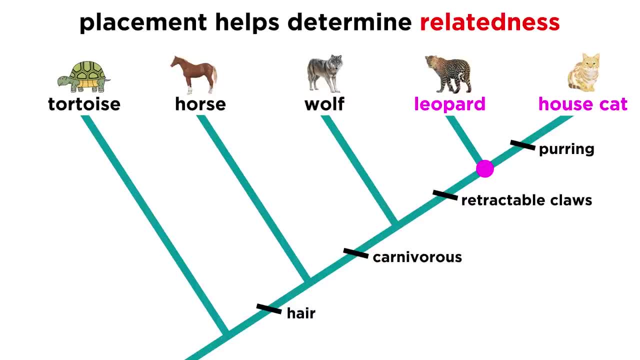 And that the leopard is more closely related to the domestic cat than to the wolf. This is fairly straightforward: Each animal listed is more closely related to the animal on its right than on its left due to their more chronologically recent common ancestry. What is somewhat less intuitive is that it doesn't always work in reverse. So domestic cats, clearly. 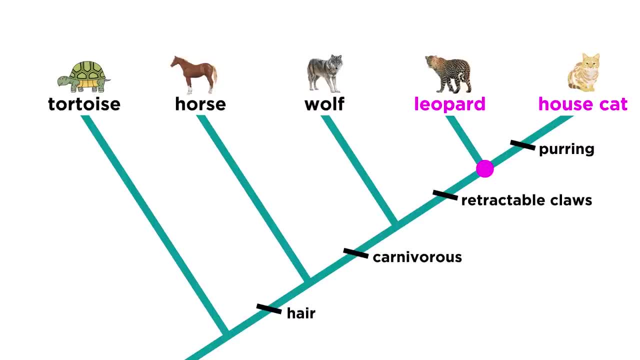 are more closely related to leopards than any other animal on the cladogram, and leopards are more closely related to domestic cats than any other animal on the cladogram. However, a horse is equally as related to a wolf as it is to a leopard, and a tortoise is equally as related. 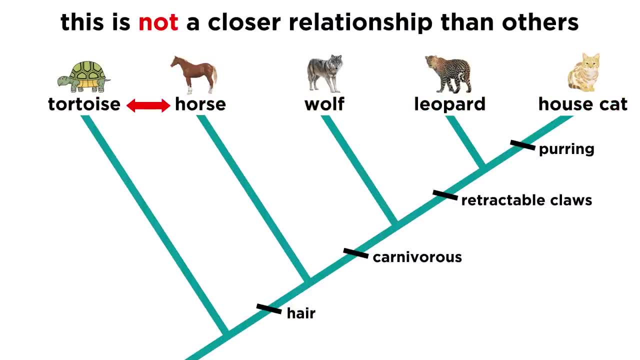 to a horse as it is a wolf. Tortoises are not more closely related to horses than to leopards, even though the cladogram might make it look like they are. Notice is that we can rewrite the cladogram any way we please, as long as each species still has. 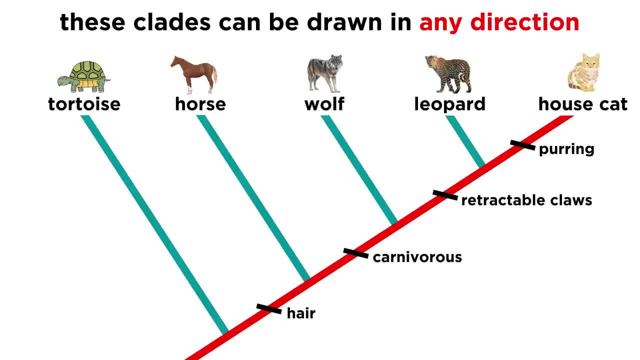 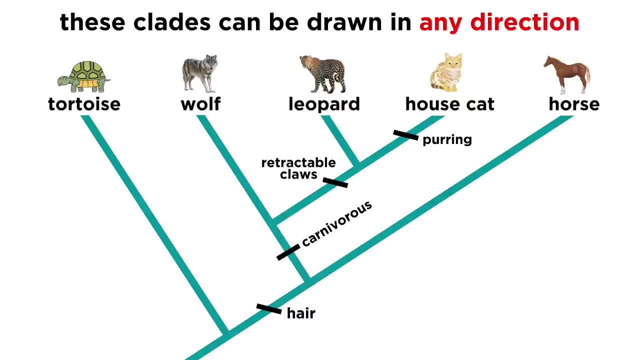 the correct characteristics. For example, even though most cladograms are written with a single line and numerous branches, we could instead write the cladogram like this, using the same characteristics. Notice that the domestic cat has the same characteristics, while the horses still. 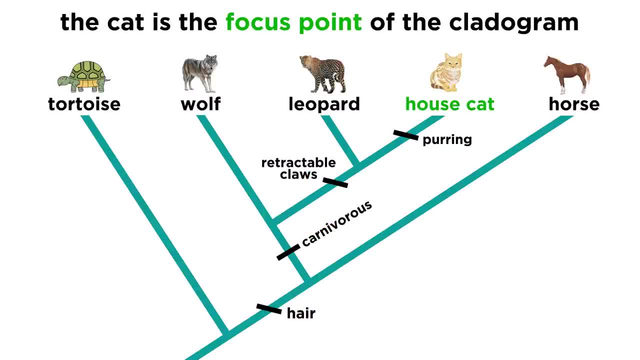 only share the characteristic of hair. This is because the domestic cat is the focus point of the cladogram, So tortoises are equally distantly related to all mammals. they're not closer to horses or cats or any other mammal in the cladogram. 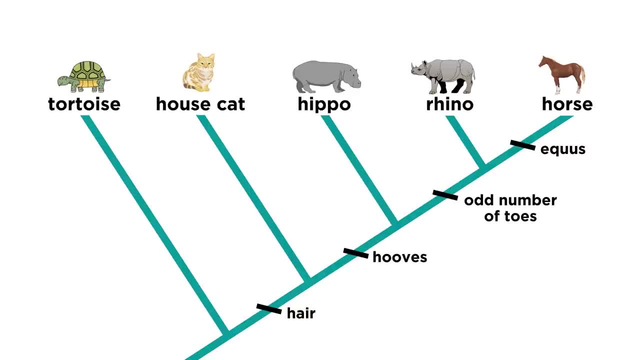 To cement this, let's rewrite the cladogram with new animals. so it looks like this Now: the horse is at the top and the domestic cat is closer to the bottom. Again, this doesn't mean anything about their evolution. Horses aren't more evolved than turtles or cats. they're just the. 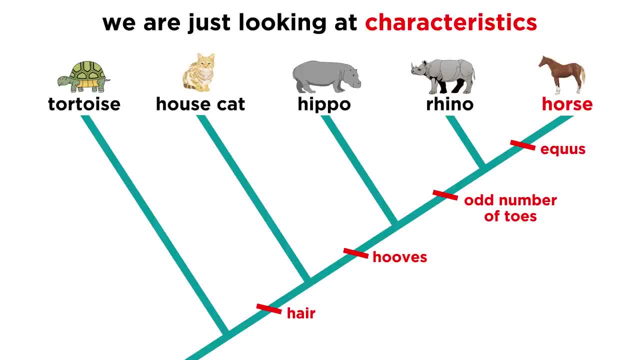 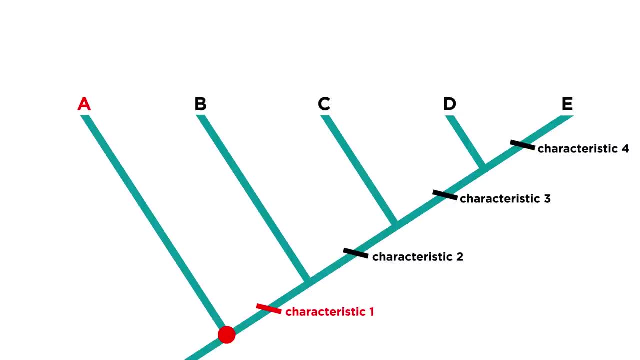 animal that possesses the greatest number of the characteristics listed on this particular cladogram. Each time an animal branches off, there is generally a characteristic listed that separates it from the others. These are known as derived characteristics. Derived characteristics shared by all members of a clade are known as synapomorphies. Going back to our original, 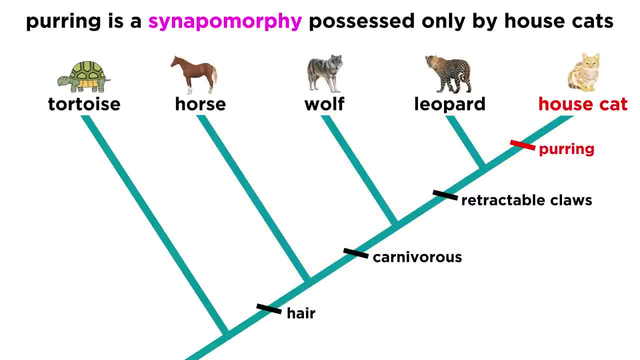 cladogram. the ability to purr is a derived characteristic Or synapomorphy that is possessed only by the domestic cat and no other animal on the cladogram. Likewise, the animals in order: carnivora, the wolf, leopard and domestic cat. 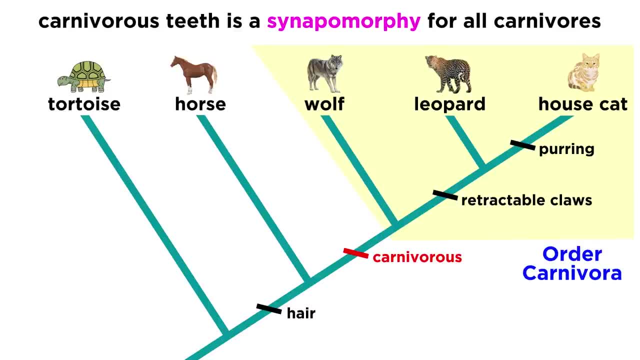 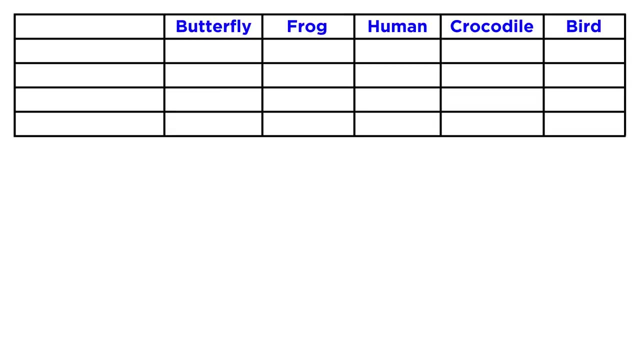 are the only animals in the cladogram with carnivorous, meat-eating teeth. Now let's try building our own cladogram. To build a cladogram, you first start with the species you're interested in studying and then determine a list of evolutionary characteristics that the 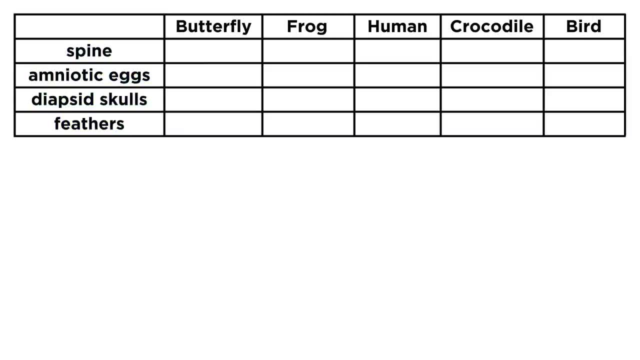 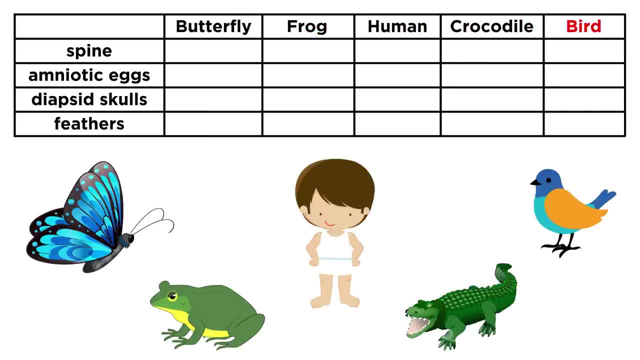 animal has. This table depicts the five organisms we will investigate, those being butterflies, frogs, humans, crocodiles and birds, as well as four characteristics, those being the presence of a spine, amniotic eggs, diapsid skulls and feathers. We can also see which of these. 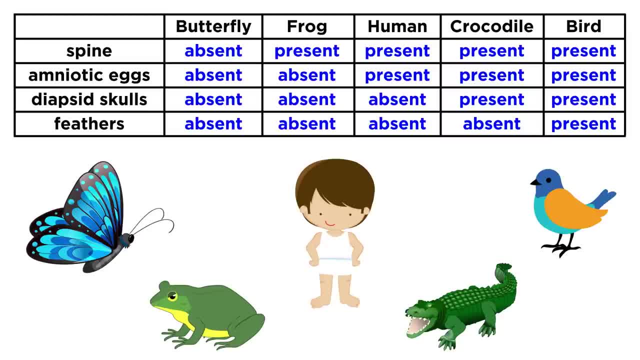 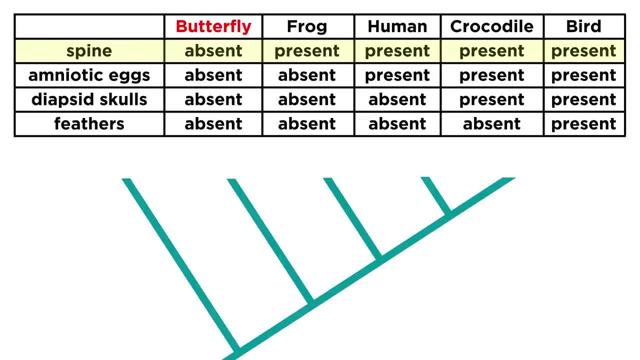 characteristics are present or absent for each organism. To make the cladogram, we observe which characteristics are more or less commonly held. For example, butterflies are the only animals out of these that do not have a spine. so let's put butterfly on the first branch and spine. 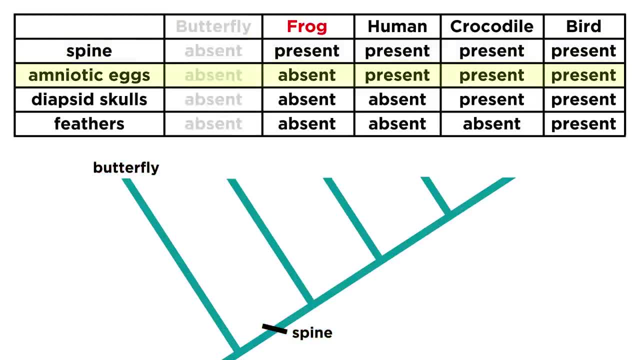 as the first characteristic Of those remaining, the only one that does not utilize amniotic eggs is the frog. so let's put the frog next and write amniotic eggs here. The rest is just the same. humans don't have diapsid skulls, so that's next. 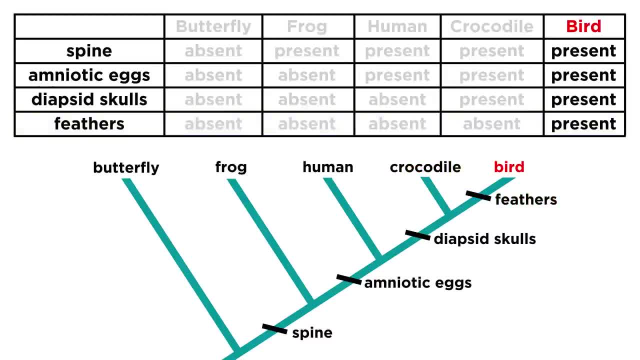 Then crocodiles do not have feathers, while birds do, which puts them at the focus point. So clearly the birds and crocodiles are the most closely related, while the butterflies are an outgroup. Looking at the cladogram, you may have some questions. Why, for example? 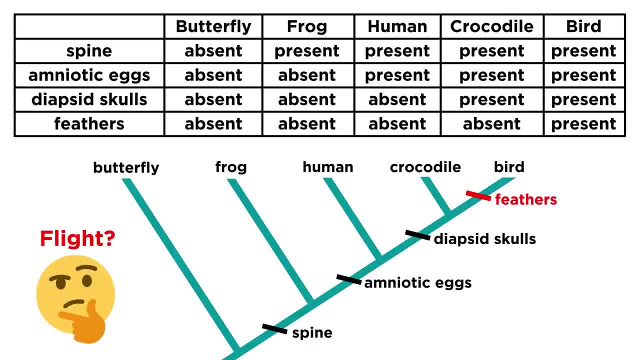 didn't we use the characteristic of flight to separate the birds from the crocodiles? Well, it is true that this is a derived characteristic of birds, but butterflies are also capable of flight, since insects convergently evolved the same characteristic. so it wouldn't be a good fit for the cladogram, since you could accidentally